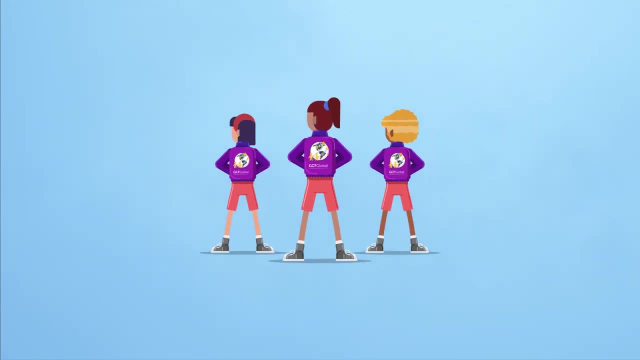 teams are having jackets made for the regional championship. The head coach wants to create a pie chart that shows which jacket sizes they'll need. She starts off by organizing the data into a table. In the first column she records the sizes Extra small, small, medium and large. 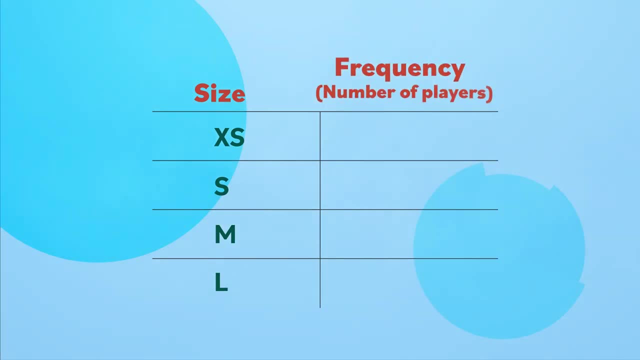 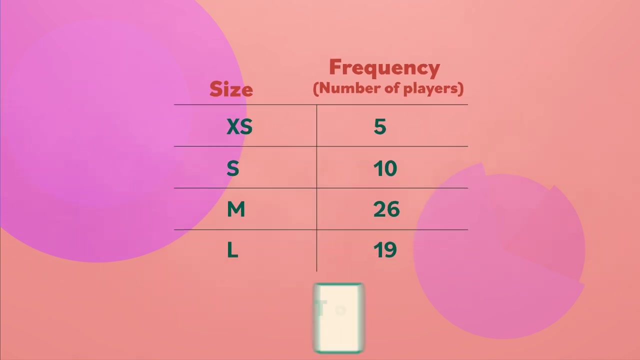 In the second column she writes down the frequency or the number of players who wear each size. Five athletes wear an extra small, Ten prefer small, Twenty-six for medium and nineteen for large. Adding up these numbers gives us the total number of players on the girls' teams: Sixty. She now needs to figure. 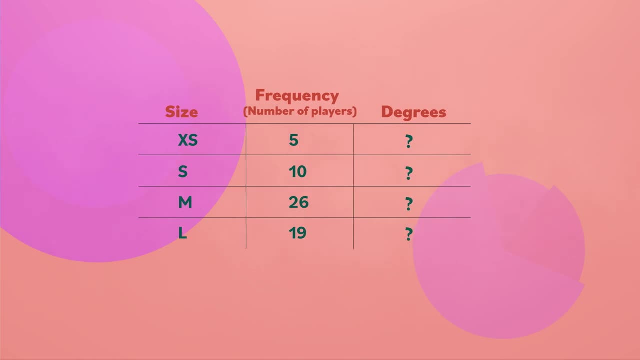 out how many degrees will each size make up in the circle of the pie chart? We know that a circle has 360 degrees. If 360 is divided by the total number of players, this tells us that one athlete equals 60. If we multiply 6 degrees by the number of players wearing each size, this tells us how big each. 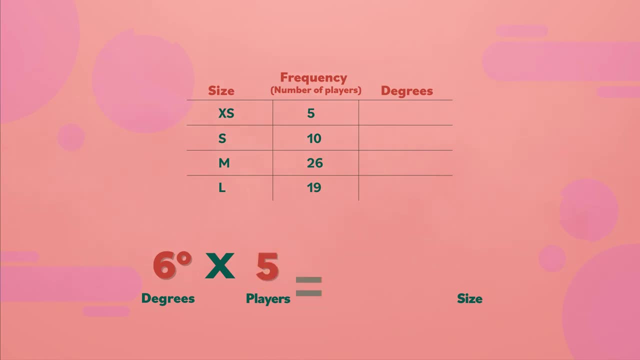 section of the pie chart should be, For example: 6 times 5 equals 30, so the extra small section should be 30 degrees in the circle. 6 times 10 is 60.. 60 degrees for size small. 6 times 26 is: 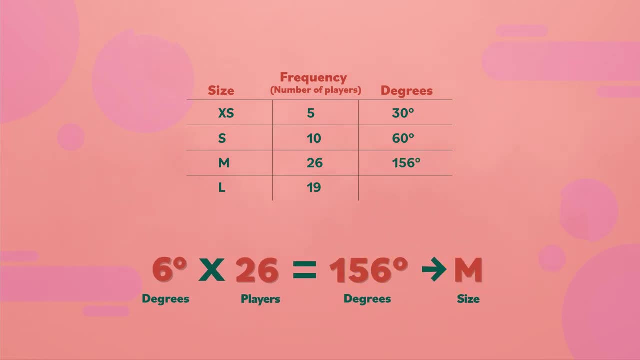 156.. Size medium will be 150 degrees. If we multiply 6 degrees by the number of players wearing each size, the total number of players will be 156 degrees. And 6 times 19 equals 114 degrees for size large. 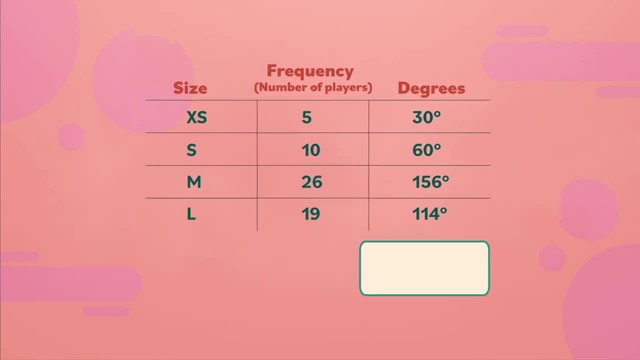 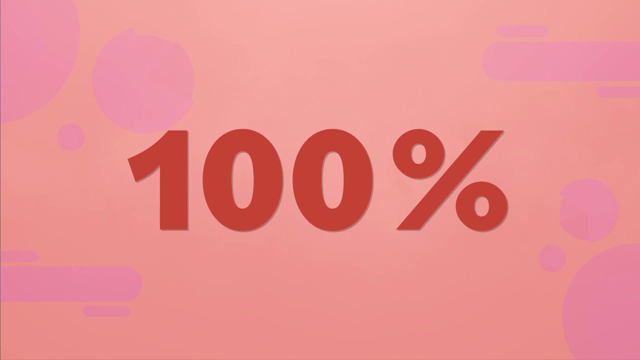 To double-check her division, the coach adds up the numbers in the degrees column. This equals 360 degrees, which means that her calculations are correct. Finally, she adds a fourth column which will show the percent of each size If 100% represents the total, and this is: 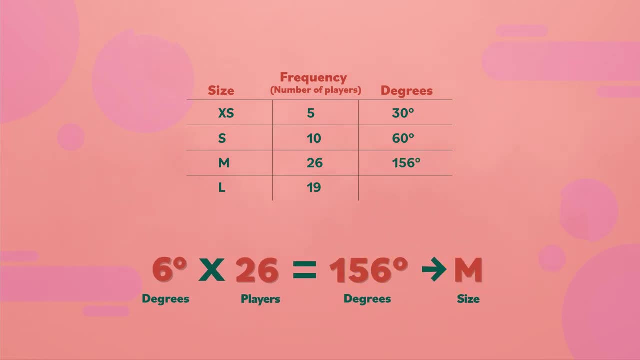 156.. Size medium will be 150 degrees. If we multiply 6 degrees by the number of players wearing each size, the total number of players will be 156 degrees. And 6 times 19 equals 114 degrees for size large. 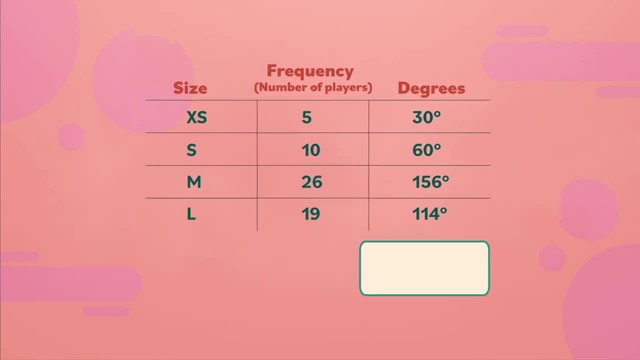 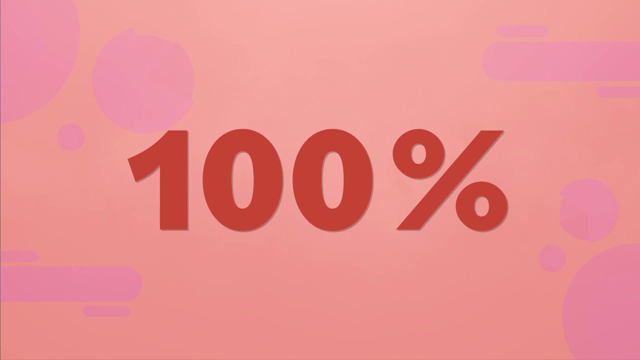 To double-check her division, the coach adds up the numbers in the degrees column. This equals 360 degrees, which means that her calculations are correct. Finally, she adds a fourth column which will show the percent of each size If 100% represents the total, and this is: 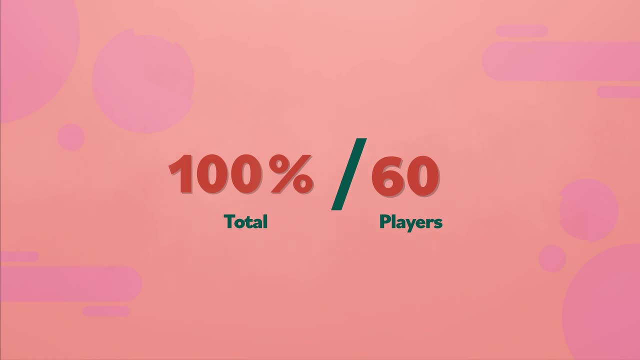 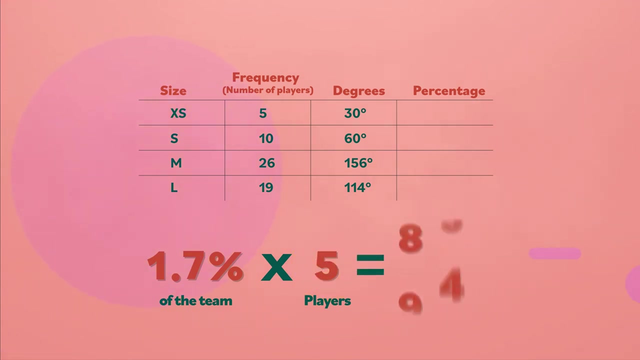 divided among 60 players, This means that each athlete equals roughly 1.7% of the team. So let's multiply 1.7 by the number of players wearing each size to determine the percentages. 1.7 times 5 equals 8.5%, 1.7 times 10 is 17%, 1.7 times 26 is 44.2% And 1.7 times 19 is. 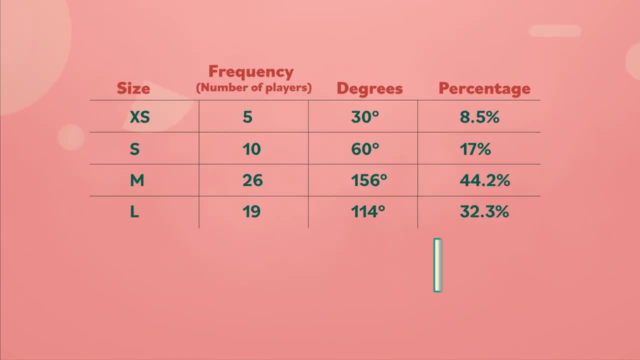 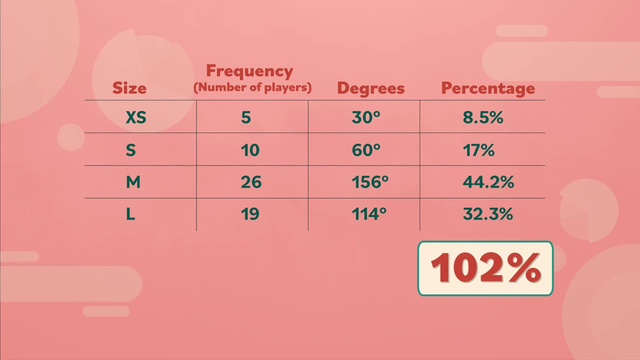 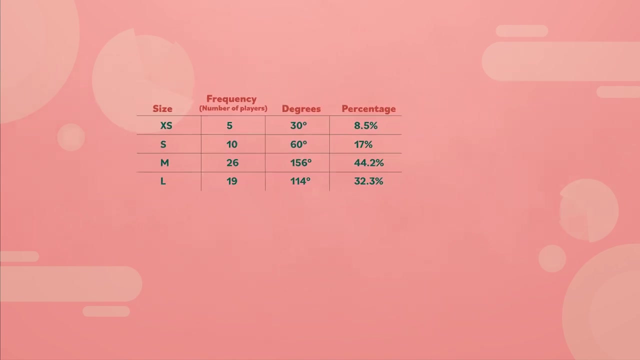 32.3%. The sum of this column should be approximately 100%. Since 1.7% was an estimate, it's OK if it goes a little over. This happens when decimals are approximated in division. Now that the table is complete, the coach begins making her graph. She traces her protractor. 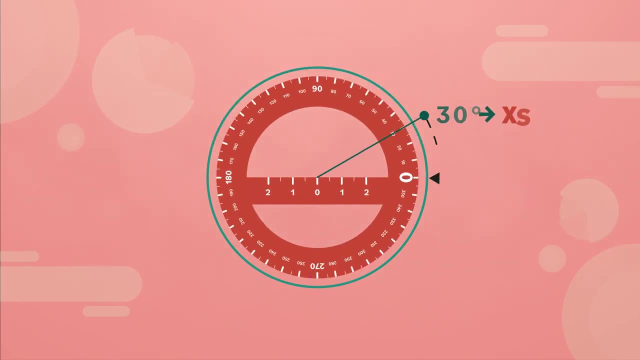 to draw a circle, then uses it to make the first 30-degree section for size extra small. We start with the first 30-degree section. The first 1.7 times 16 is 32.2.. The next one is 6.5%. The next one is 6.8 times 4.3.. The next one is 6.8%. The next one is 4.3.. The next one is: 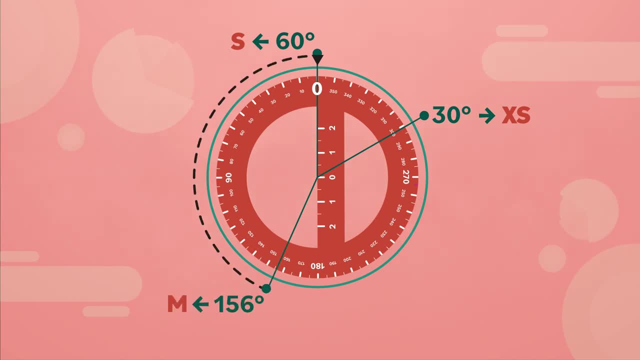 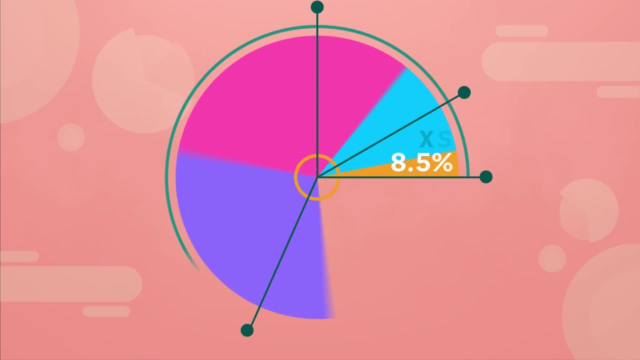 for size small, 156 degrees for size medium and 114 degrees for size large. Finally, she adds the percentage to each slice of the pie, making the chart easier to read. Feel free to check out our other videos about statistics or the full. 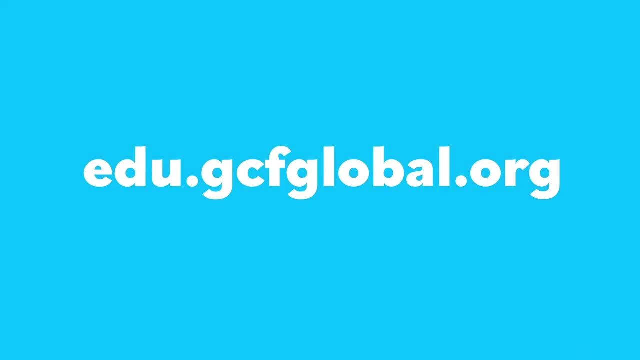 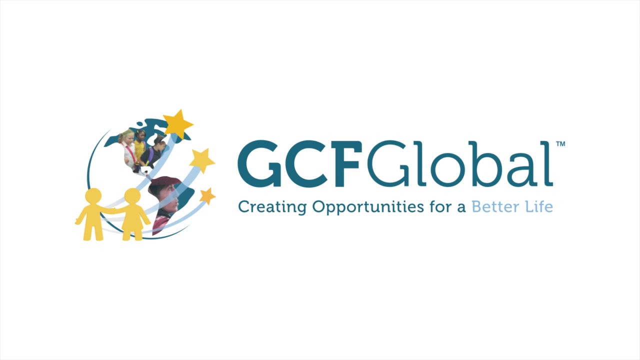 tutorial on our website at GCFGlobalorg. GCF Global: Creating opportunities for a better life.